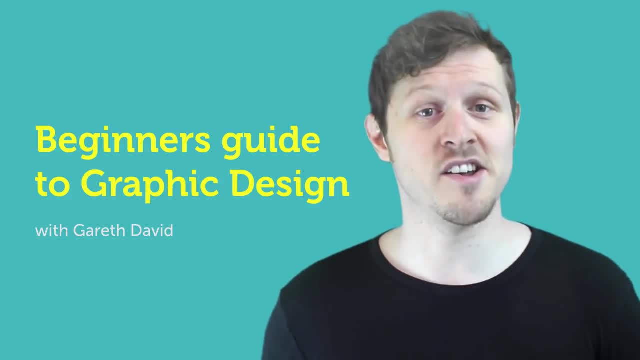 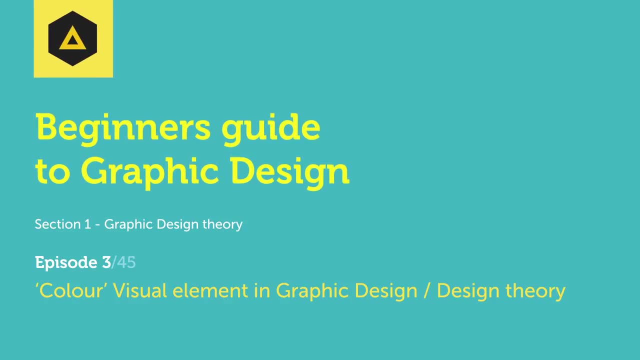 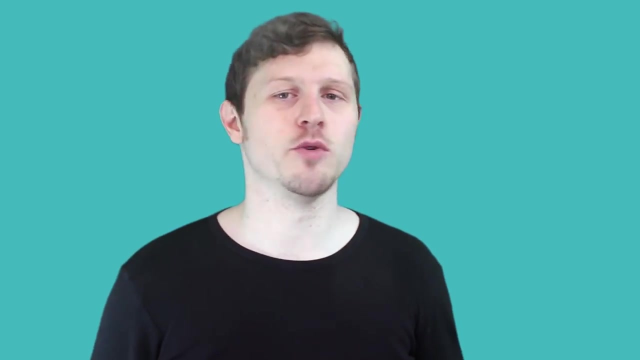 becoming a graphic designer, then join me as I discuss a series of graphic design topics. So the graphic part of graphic design is made up of visual elements, the building blocks of design. Through the harness of our artistic expression, we choose these visual elements and arrange them on. 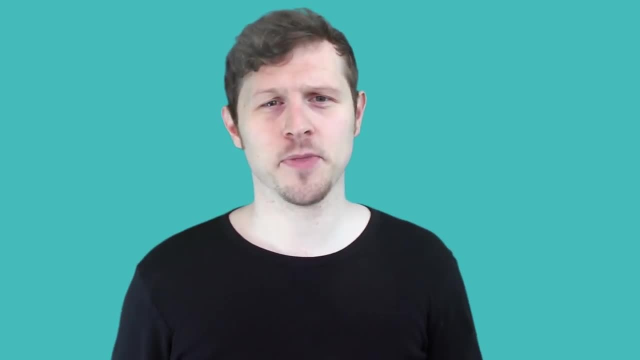 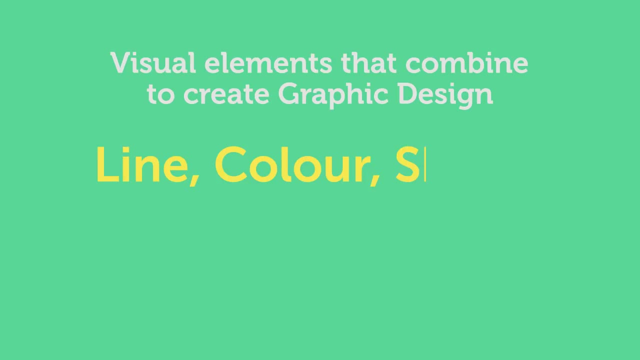 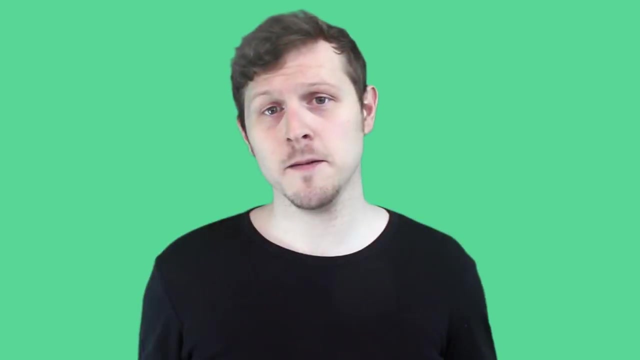 a surface in a layout to convey an idea. The basic visual elements that combine to create graphic design include the following: Line, color, shape, texture, space, form and typography. Whatever work you produce, be it for a magazine, a poster, a website or advertisement. 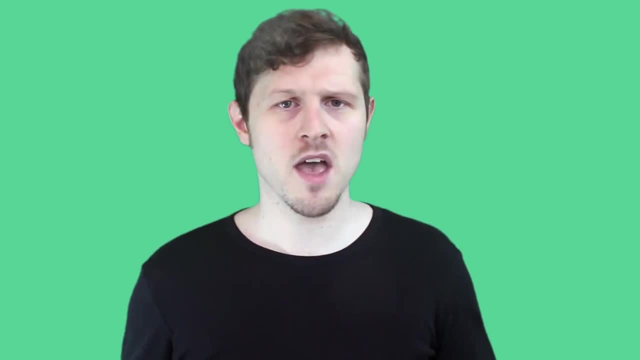 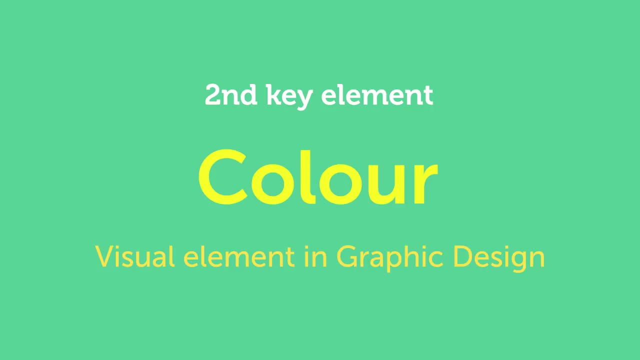 these visual elements will play a part in your design. In this video, I'm going to discuss the second key visual and discuss color as a visual element in graphic design. In this video, I will be referring to some visual diagrams. If you wish to follow along, you can download the pdf. 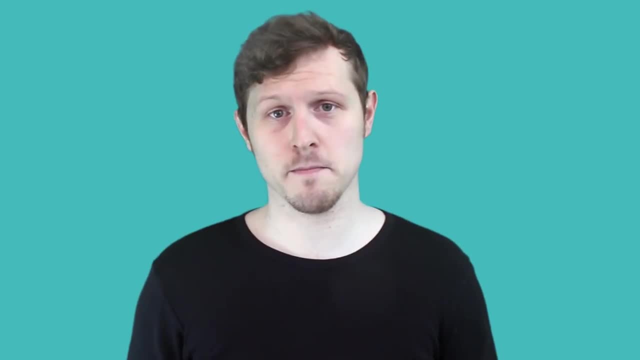 document that accompanies this series Link is in the description. So color plays one of the biggest roles in graphic design. It can give emphasis, it can be used as a mechanism of organization, it can create impact and create a specific look and feel in a piece of graphic design. 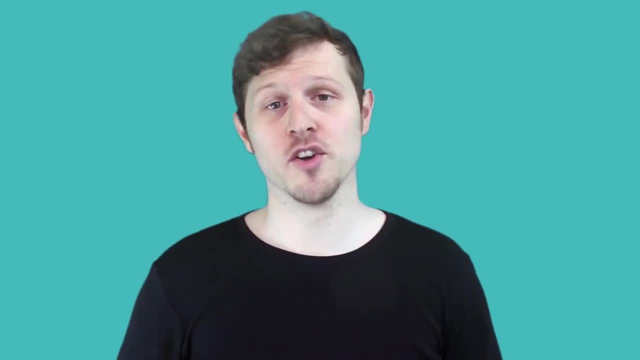 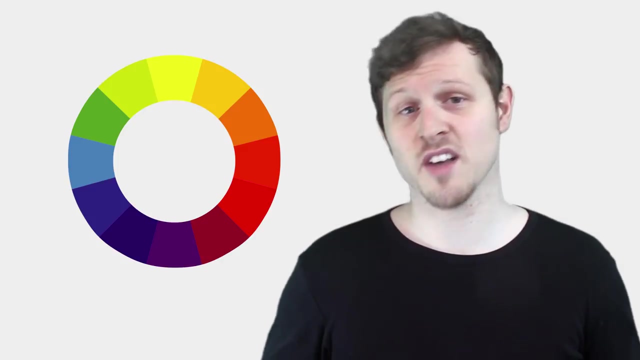 work. When working with color, it helps to have a good knowledge of color theory. Color theory provides us with practical guidance to help us mix colors and create interesting color combinations. And it all starts with the color wheel. The color wheel is a really useful tool designed to help us. 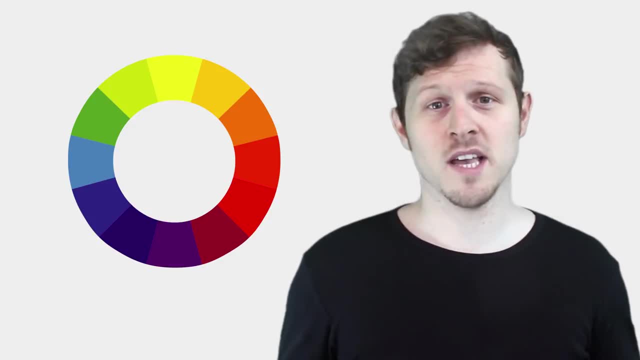 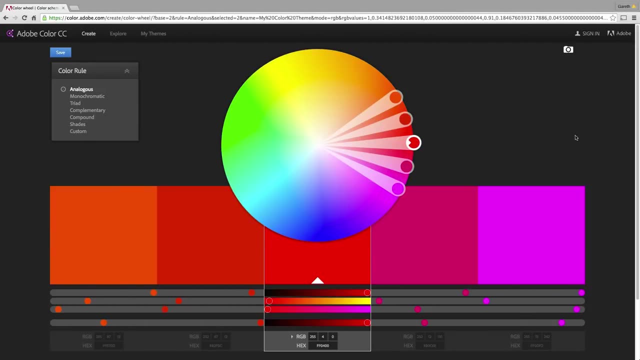 identify colors that work well together. So this year is the red, yellow, blue color model, which consists of 12 colors. Now if we jump onto the Adobe color website, we can see this color wheel as more of a spectrum. This is an amazing resource to explore and create color schemes. The address: 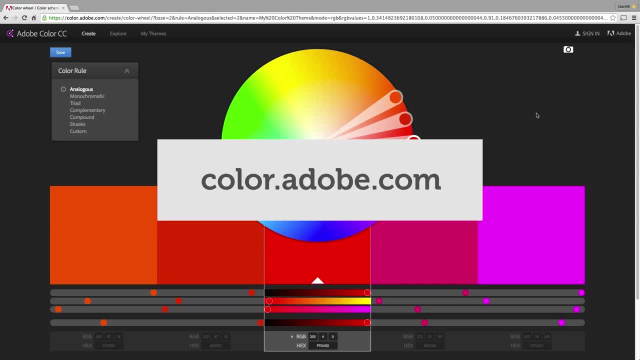 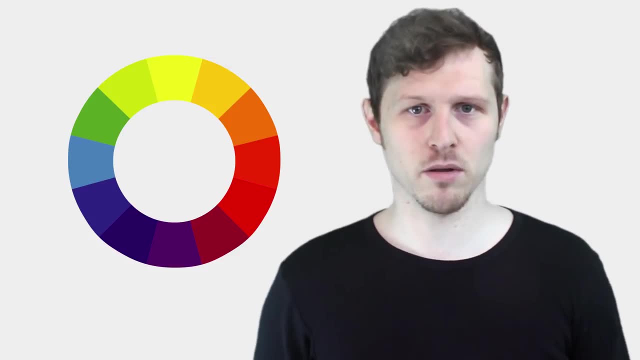 for this website is coloradobecom. I'll be referring to this website later in this episode, but for now, to help explain color theory, I'll use this simple example. If you want to take a closer look at this color wheel and the spectrum, you can find them in the downloadable PDF. Link is in the description. 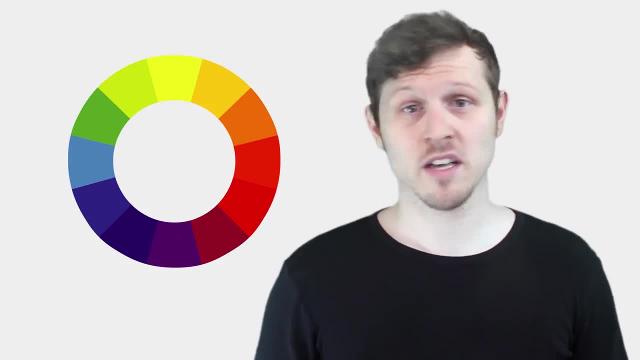 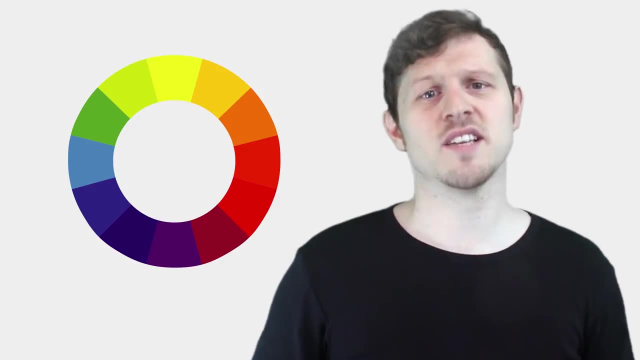 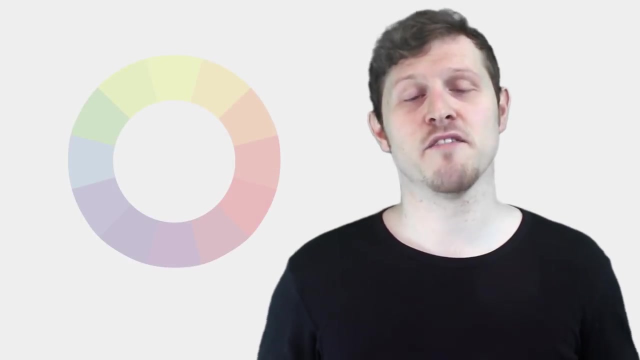 So the color wheel consists of primary colors, secondary colors and tertiary colors, and these can be split into warm and cool colors. So let's take a look at each of these. So first is primary colors. Primary colors make up the basis for the color wheel. Here they are. 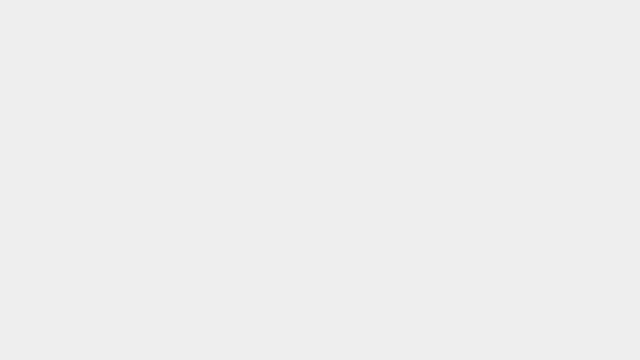 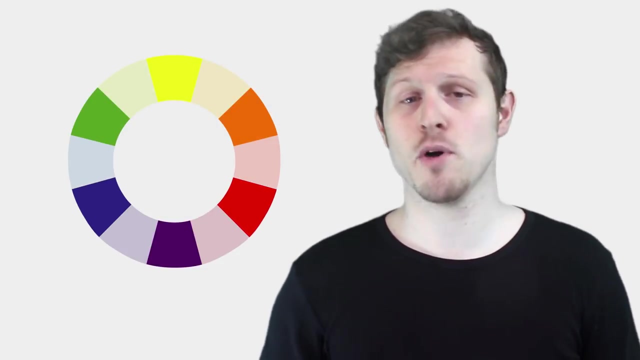 red, yellow and blue. Next are the secondary colors. Secondary colors are made by mixing equal portions of the primary colors. These create green, orange and purple. Next are the tertiary colors. Tertiary colors are made by mixing a primary color with a neighboring. 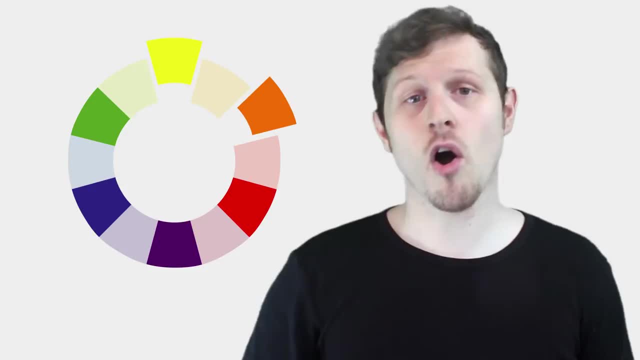 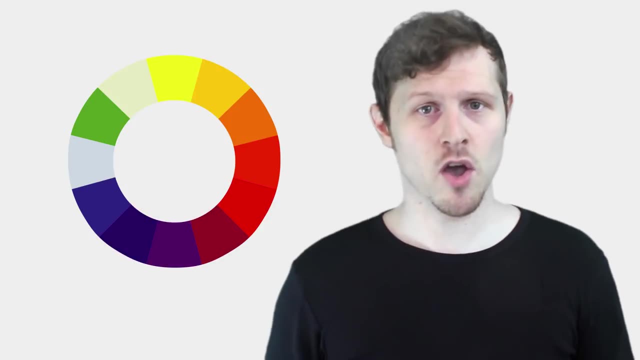 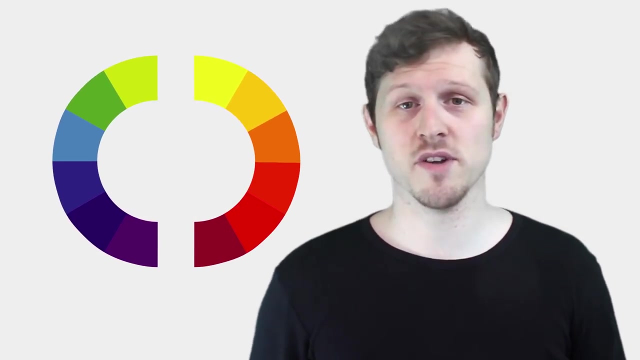 secondary color. For example, if we mix the yellow with the orange, we get a yellowy orange color in between. If we continue to mix the primary and neighboring colors, we fill the gaps in the color wheel. We get the remaining tertiary colors. Now, if we separate the color wheel, we get two categories. 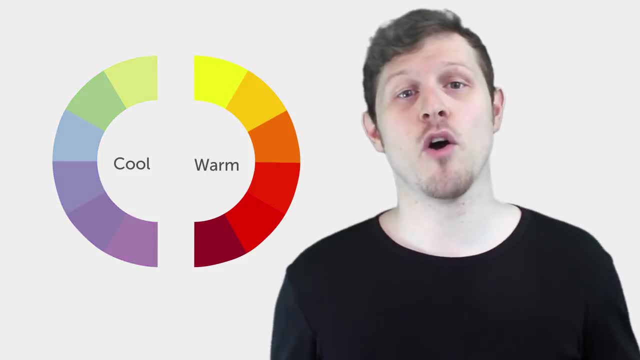 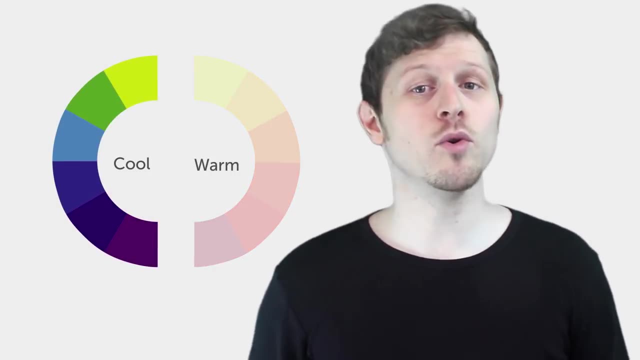 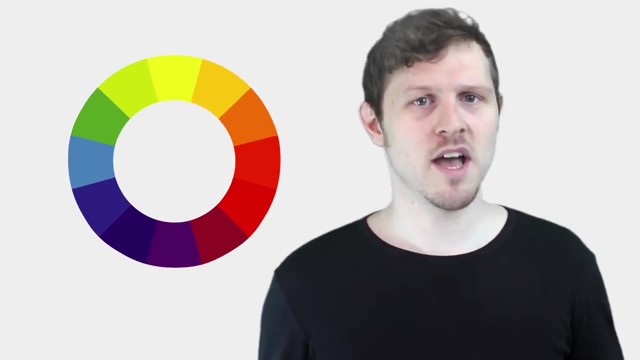 warm and cool colors. On the right we have the warm colors. These incorporate the red, violet colors through to yellow. On the left, we have cool colors. These incorporate the colors yellow through to indigo. So that completes the color wheel. Now this is a really useful tool. 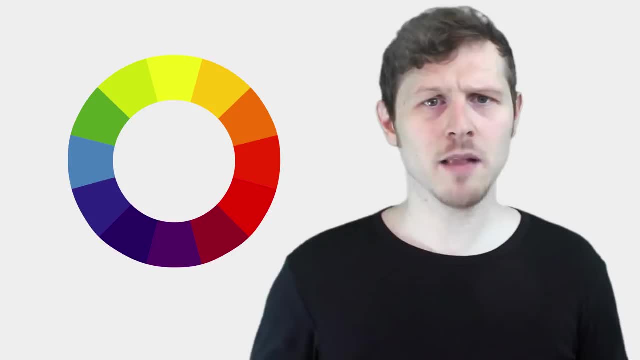 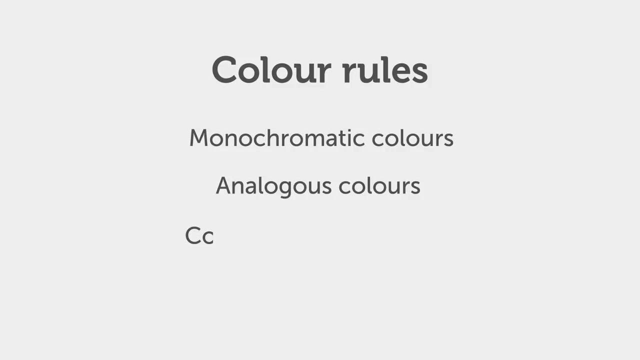 designed to help us choose color schemes, To help us choose interesting color combinations that have harmony together or create contrast. there are some color rules we can explore. These color rules are referred to as monochromatic colors, analogous colors, complementary colors and triadic colors. So first we have monochromatic colors. 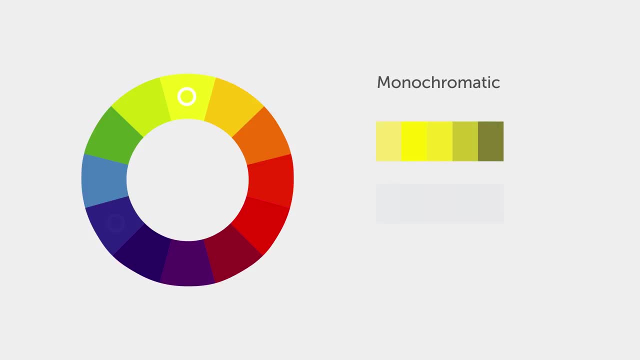 Monochromatic colors are shades and tints of the same color. The monochromatic color scheme is typically balanced and easy on the eye. Now, if we jump onto the adobe color website at coloradobecom, we can see some of these color rules on the left. 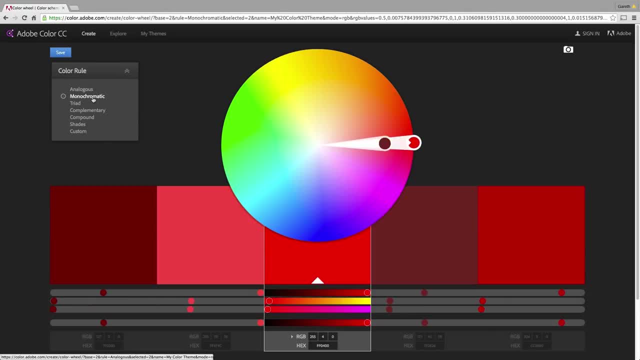 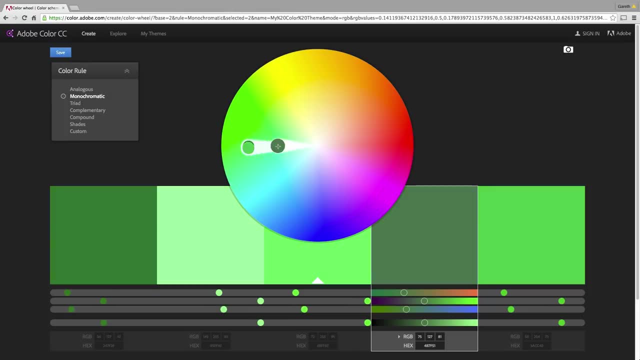 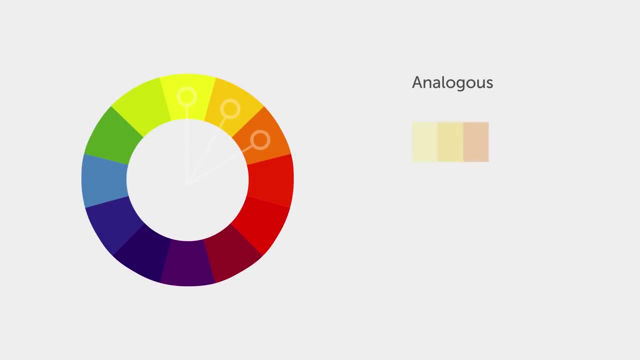 If I click on the monochromatic, it will generate a monochromatic color scheme below. Now, if I click and drag the middle color circle in the spectrum and toggle the others, it will generate new schemes. Next we have analogous colors. Analogous colors are those found close to each.